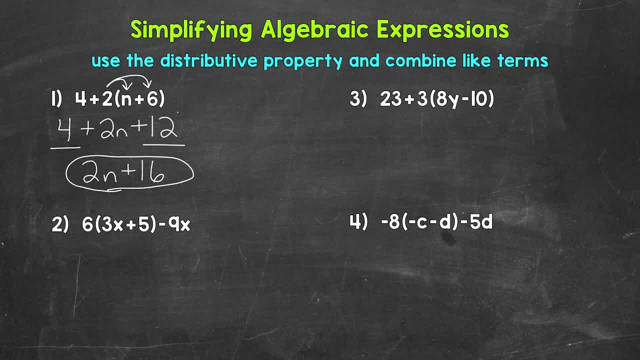 variables. they go in order From greatest to least as far as exponents, And then, if variable terms have the same exponents, go in ABC order. So again for number one, we just have two terms: a variable term and then 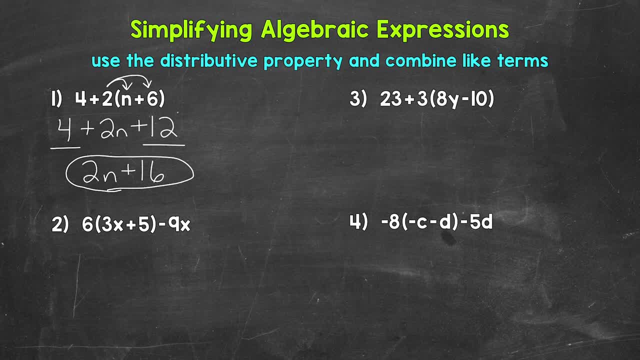 a constant term. So 2n plus 16 is our final simplified expression. Now that final simplified expression is equivalent to the original expression. We were just able to simplify that original expression by using the 2n plus 16. So we can look to combine like terms to. 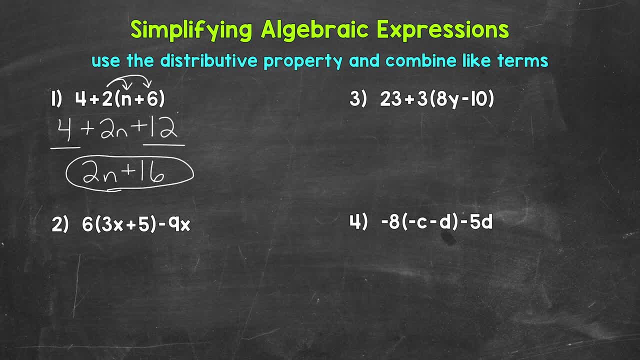 solve this problem. Let's move on to number two, where we have 6 and then, in parentheses, 3x plus 5 and parentheses minus 9x. Let's start by using the distributive property to remove the parentheses. So let's distribute this 6 to the 3x and to the 5.. 6 times 3x gives us 18x, And then 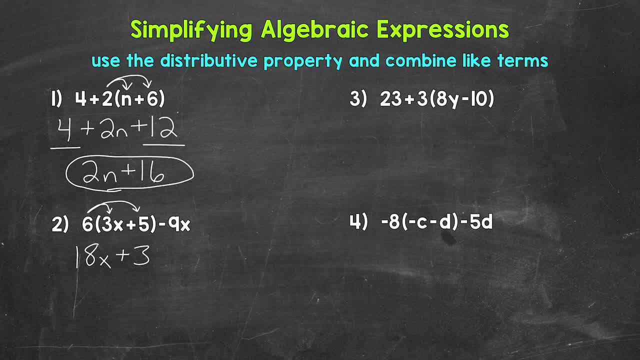 6 times 5 gives us a positive 30. So plus 30. Then we have minus 9x, So a negative 9x. Now that we removed the Parentheses we can look to combine like terms 18x and negative 9x. 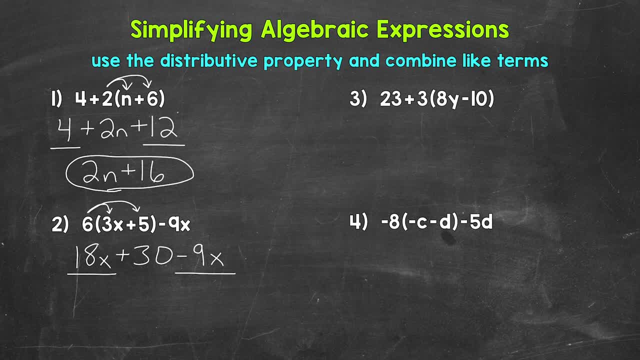 are like terms so we can combine them. Make sure to include the sign that's in front of a term that is negative 9x, So we have 18x plus 3x, plus seven, six, 258.. I always review these four things as common termsativa. Mod範 crem jei cube. 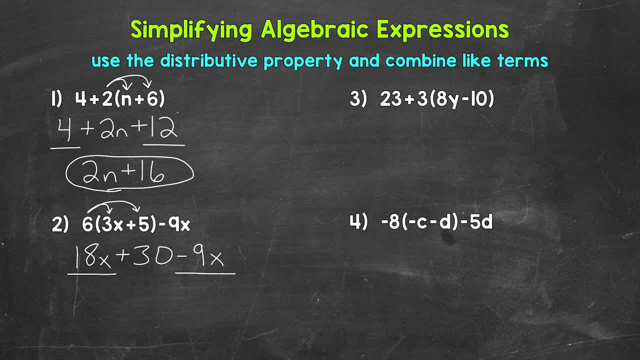 So we have 18x minus 9x or 18x combined with negative 9x. That gives us a positive 9x, and then we have plus 30, a positive 30. So our final simplified expression is 9x plus 30. 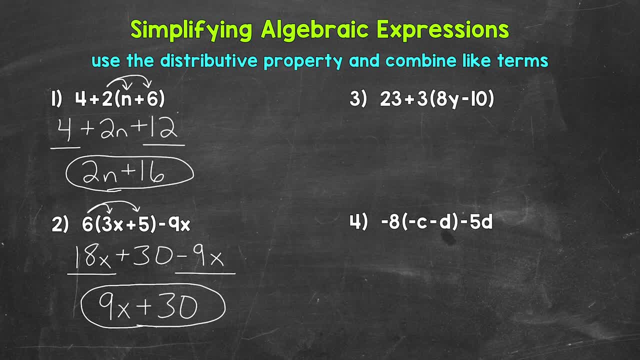 Let's move on to number 3, where we have 23 plus 3, and then, in parentheses, 8y minus 10.. Let's remove the parentheses by using the distributive property. So let's distribute the 3 to the 8y and to the negative 10.. 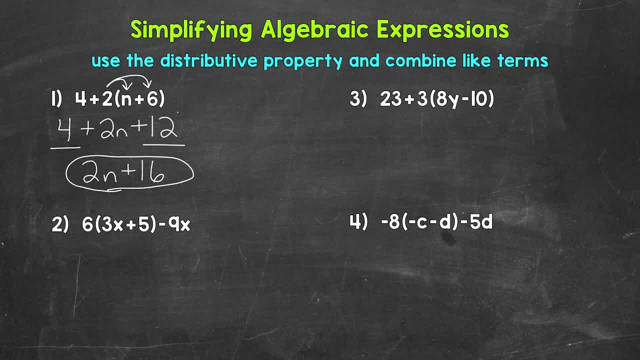 variables. they go in order From greatest to least as far as exponents, And then, if variable terms have the same exponents, go in ABC order. So again for number one, we just have two terms: a variable term and then 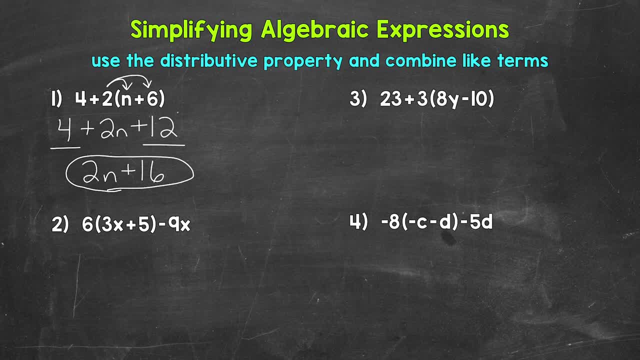 a constant term. So 2n plus 16 is our final simplified expression. Now that final simplified expression is equivalent to the original expression. We were just able to simplify that original expression by using the 2n plus 16. So we can look to combine like terms to. 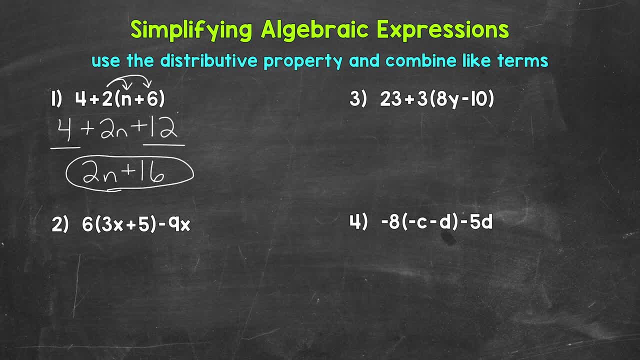 solve this problem. Let's move on to number two, where we have 6 and then, in parentheses, 3x plus 5 and parentheses minus 9x. Let's start by using the distributive property to remove the parentheses. So let's distribute this 6 to the 3x and to the 5.. 6 times 3x gives us 18x, And then 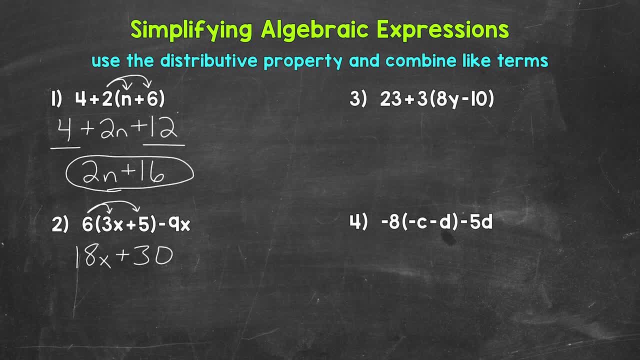 6 times 5 gives us a positive 30. So plus 30. Then we have minus 9x, So a negative 9x. Now that we removed the parentheses we can look to combine like terms 18x and negative. 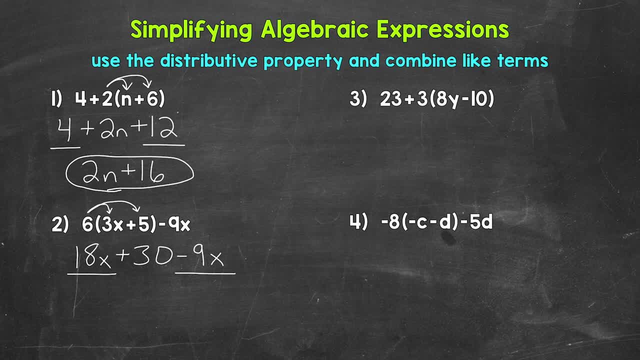 9x are like terms So we can combine them. Make sure to include the sign that's in front of a term. That's negative 9x. So we have 18x minus 9x or 18x combined with negative 9x. That gives us a positive 9x. and then we have 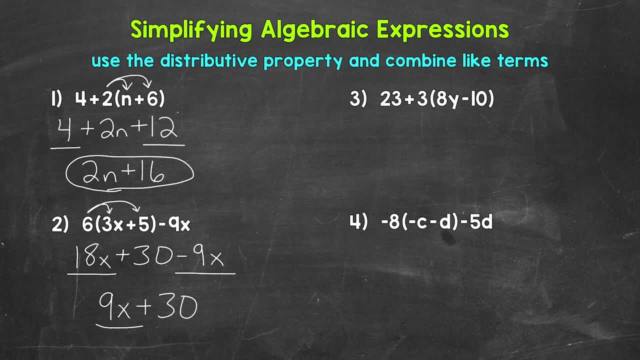 plus 30, a positive 30. So our final simplified expression is 9x plus 30.. Let's move on to number 3, where we have 23 plus 3, and then, in parentheses, 8y minus 10.. Let's remove the parentheses by using: 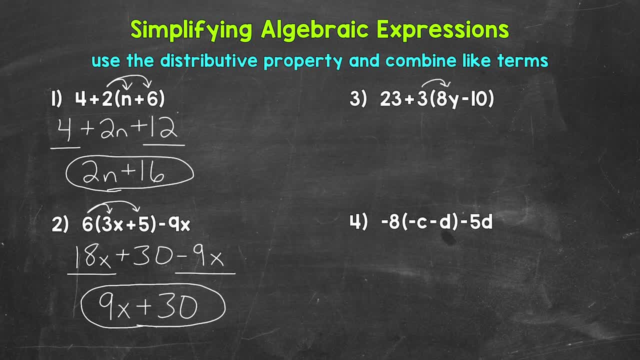 the distributive property. So let's distribute the 3 to the 8y and to the negative 10.. 3 times 8y gives us 24y, and then 3 times negative 10 gives us negative 30. This is a positive. 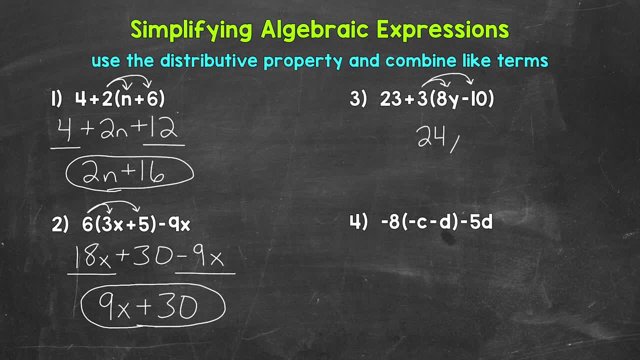 3 times 8y gives us 24y, and then 3 times negative 10 gives us negative 30. This is a positive 24y, and then bring down the 23.. Now, as far as the distributive and subtraction, we can also think through that as 3 distributed to 8y. 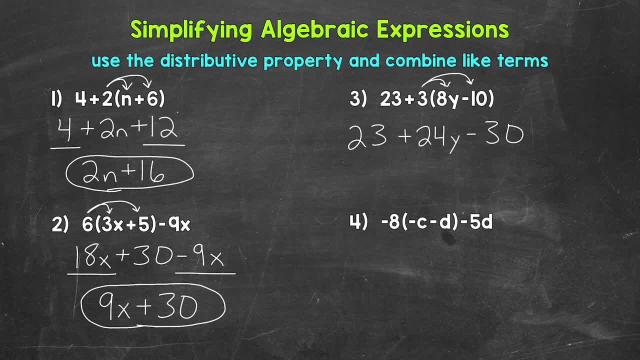 So 3 times 8y, that gives us 24y. Then we can bring the subtraction sign down and then distribute the 3 to the 10.. So 3 times 10,, that gives us 30. So 24y minus 30.. 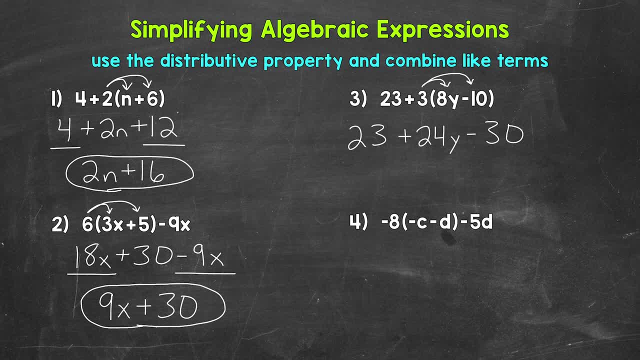 We got the same thing thinking through the distributive property that way as well. Now that we removed the parentheses, we can look to combine like terms. We have two constant terms, 23 and negative 30. So we can combine those like terms. 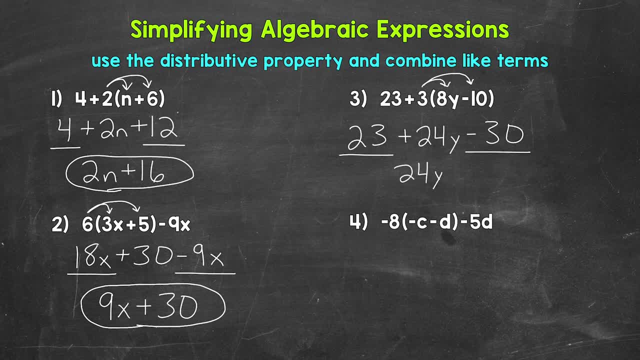 So we have 24y, and then 23 minus 30, or 23 combined with negative 30, gives us negative 7,, so minus 7.. Our final simplified expression: 24y minus 7.. Lastly, let's move on to number 4, where we have negative 8,. 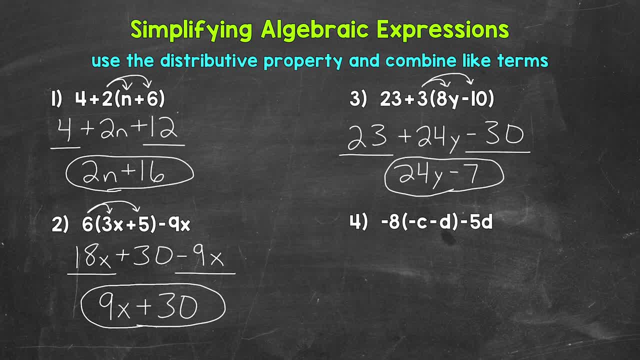 and then in parentheses, negative c minus d and parentheses minus 5d. Let's start by removing the parentheses by using the distributive property. Distribute the negative 8 to the negative c and distribute the negative 8 to negative d. 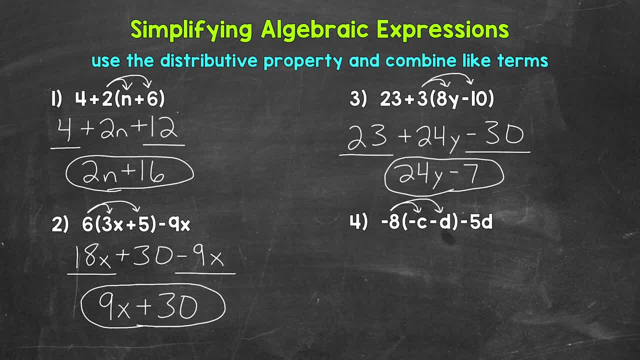 Negative 8 times negative. c gives us a positive 8c. Remember a negative times a negative equals a positive. Negative 8 times negative. d gives us a positive 8d. And then we have minus 5d, so a negative 5d. 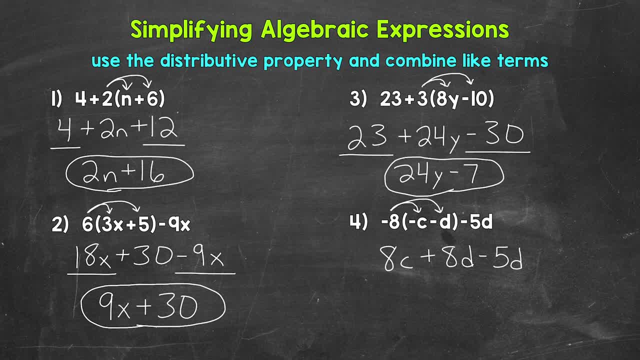 Now that we removed the parentheses, we can look to combine like terms: 8d and negative 5d are like terms, So we can look to combine like terms: 8d and negative 5d are like terms, So we can look to combine like terms: 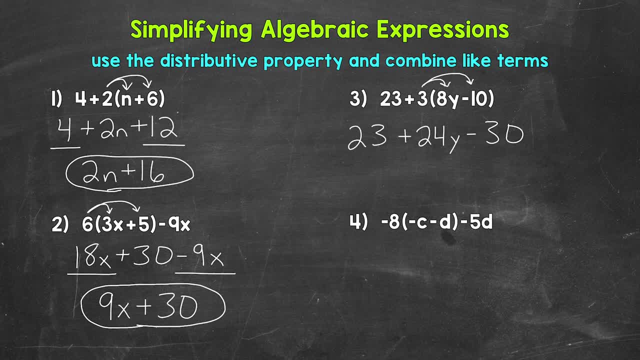 24y and then bring down the 23.. Now, as far as the distributive property and subtraction, we can also think through that as 3 distributed to 8y, so 3 times 8y, that gives us 24y. Then we can. 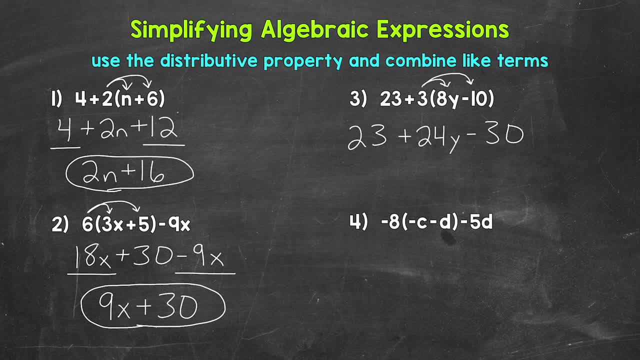 bring the subtraction sign down and then distribute the 3 to the 10. So 3 times 10, that gives us 30. So 24y minus 30. We got the same thing thinking through the distributive property that way as well. Now that we removed, 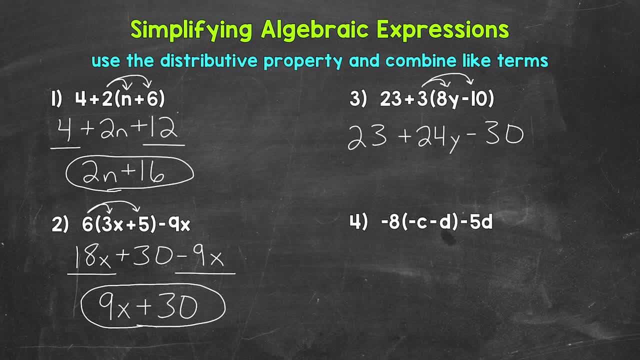 the parentheses. we can look to combine like terms. We have two constant terms, 23 and negative 30. So we can combine those like terms. So we have 24y and then 23 minus 30, or 23 combined with. 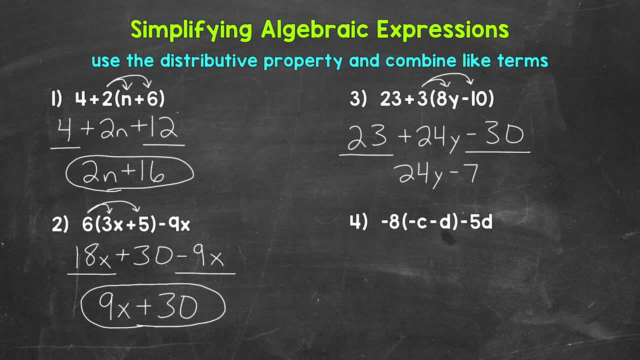 negative 30, gives us negative 7.. So 24y minus 7.. Our final simplified expression: 24y minus 7.. Lastly, let's move on to number 4, where we have negative 8, and then, in parentheses, negative c minus d. end parentheses. 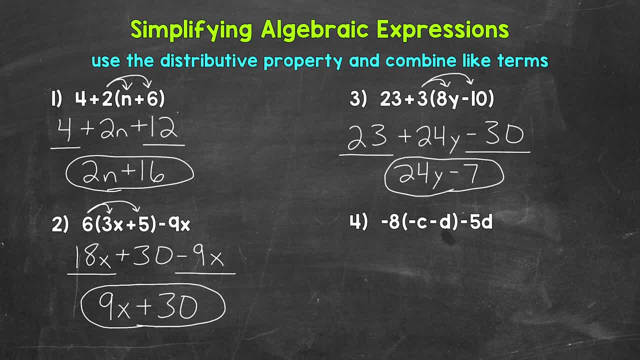 minus 5d. Let's start by removing the parentheses by using the distributive property. Distribute the negative 8 to the negative c and distribute the negative 8 to the negative c and distribute the negative 8 to the negative c. 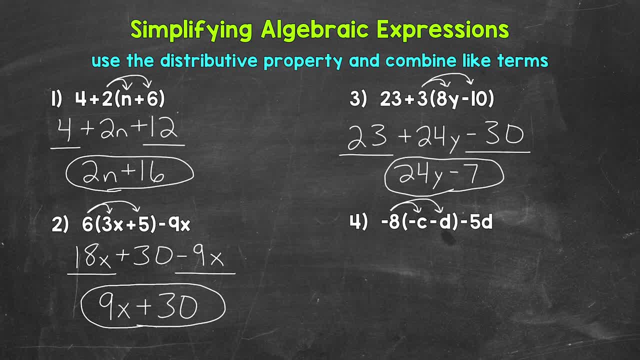 and distribute the negative 8 to the negative d. Negative 8 times negative c gives us a positive 8c. Remember: a negative times a negative equals a positive. Negative 8 times negative d gives us a positive 8d. And then we have minus 5d, so a negative 5d, Now that we removed the parentheses. 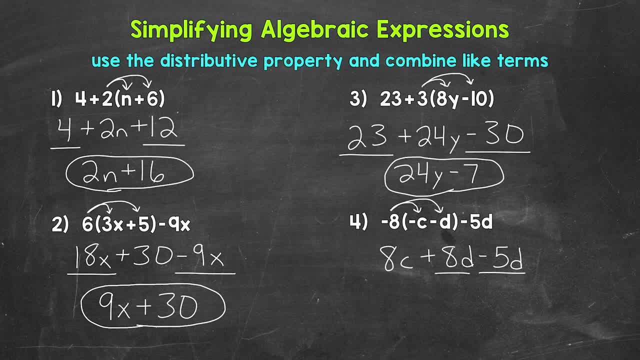 we can look to combine like terms. 8d and negative 5d are like terms, So let's combine those like terms. We end up with 8c and then 8d minus 5d or 8d combined with negative 5d.